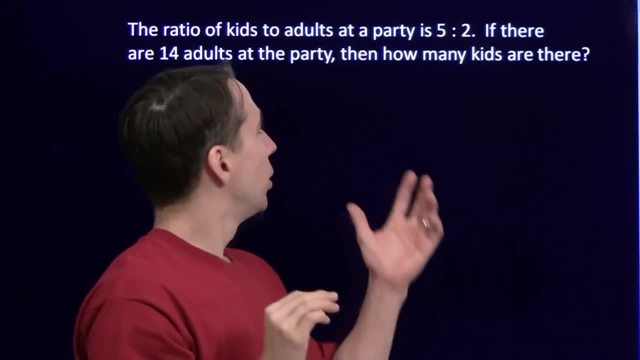 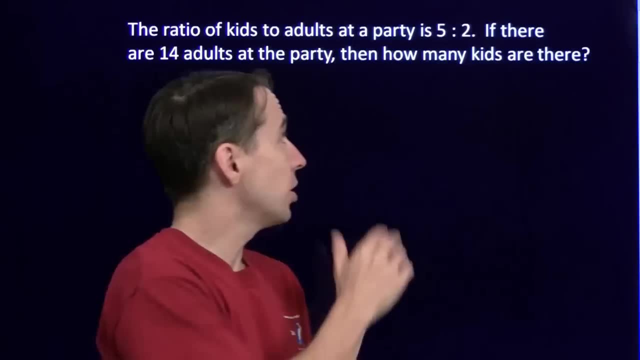 And that's the ratio. What the ratio means is that for every 5 kids at the party, there are 2 adults at the party. It doesn't tell us how many people are at the party. The ratio doesn't tell us how many kids there are. It doesn't tell us how many adults there. 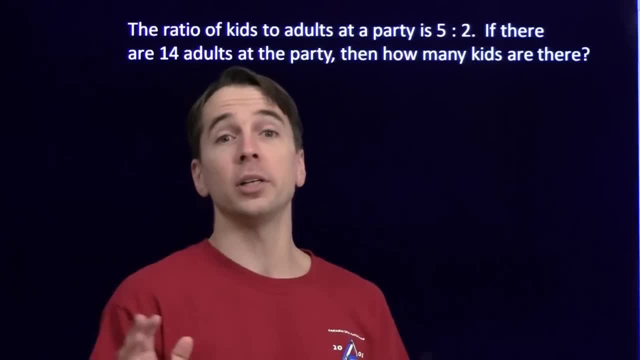 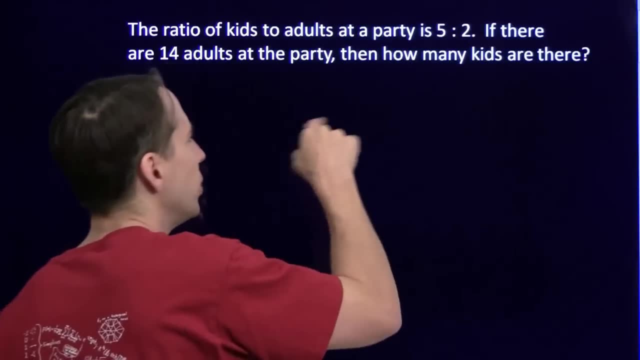 are. It just tells us that for every 5 kids there are 2 adults. We can put everyone in the party in groups and each of those groups will have 5 kids, 2 adults. That's all this ratio tells us. It doesn't tell us how many groups there are. Let's read the rest of the 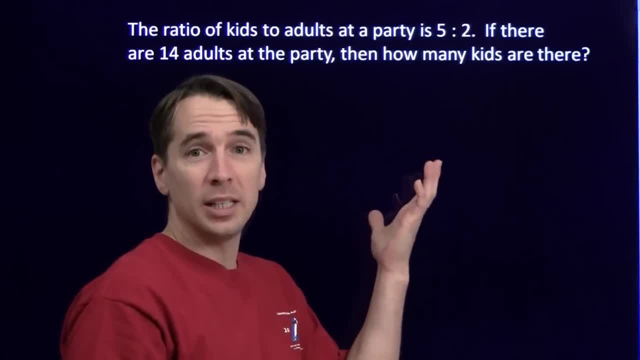 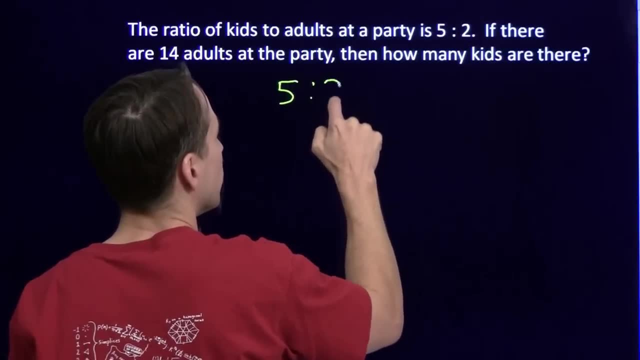 problem here. It says: if there are 14 adults at the party, then how many kids are there? So our ratio here tells us that we have 5 kids for every 2 adults. We could just have 5 kids and 2 adults, and that's it. Or we could have 2 of those groups If we had 2. 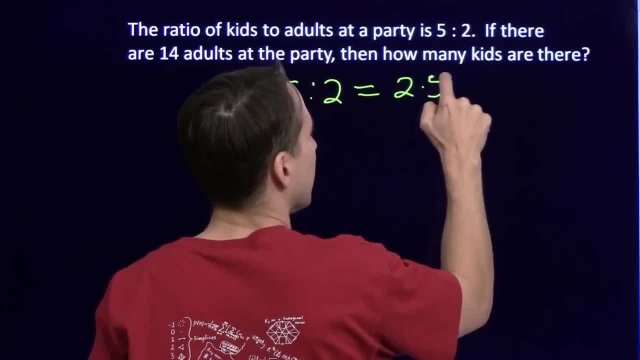 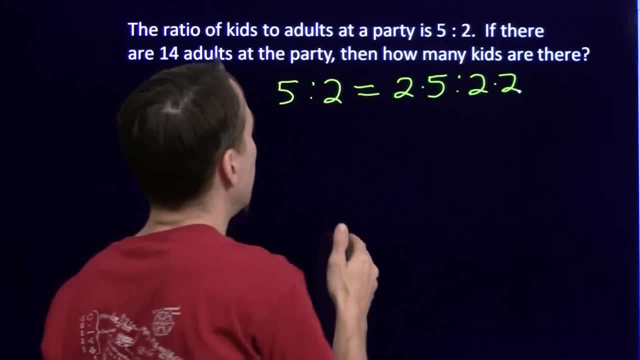 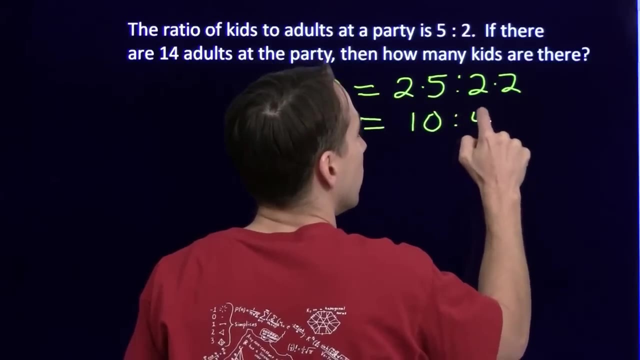 of those groups. well then, we'd have 2 times 5 kids and 2 times 2 adults, And all we're doing here is multiplying each of these components, each of these parts of the ratio, by 2.. So if we had 2 of these groups, that will give us 10 to 4.. 10 kids, 4 adults. 4 isn't 14.. 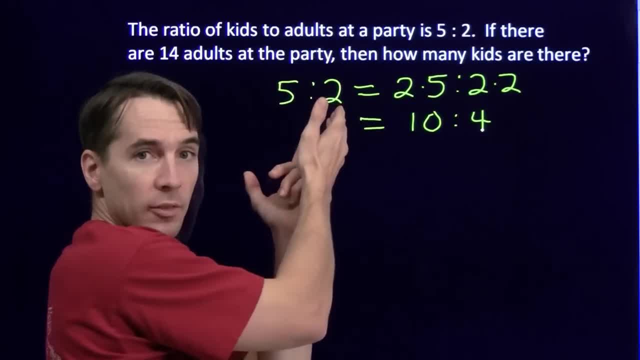 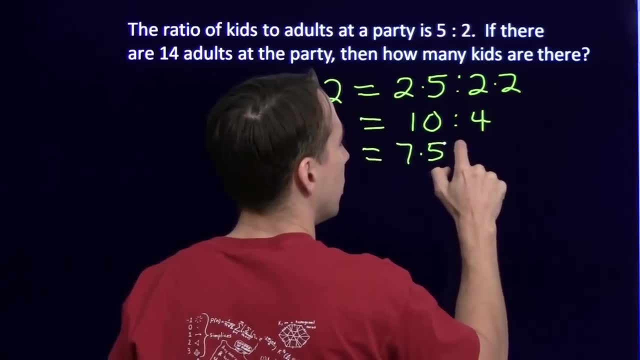 In order to get to 14 adults. well, we need 7 of these groups, 7 of these groups of 2.. So we can take a group of adults and we're going to multiply each of these groups by our ratio And again, multiply both parts by the same number. Multiply them both by. 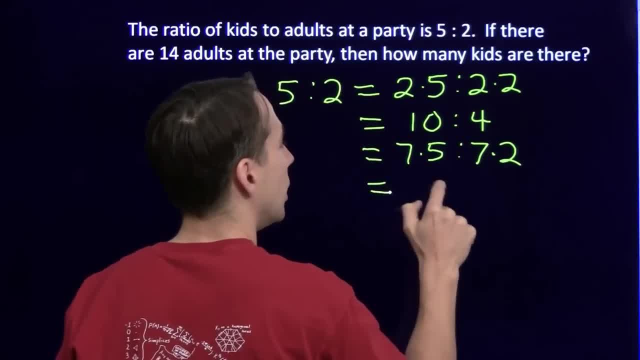 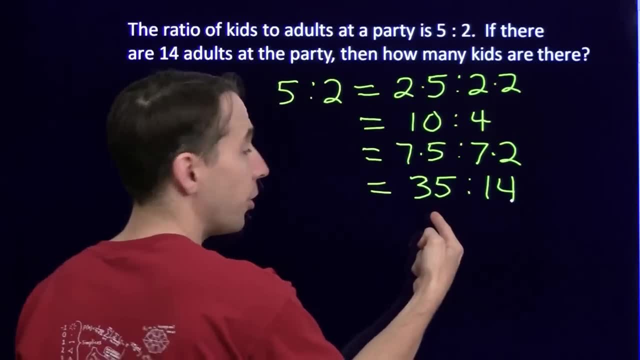 7. now It's like taking 7 of these groups and we get 35 to 14.. 14 adults, 35 kids. So we've answered the problem. We know there are 35 kids at the party And what we're doing. 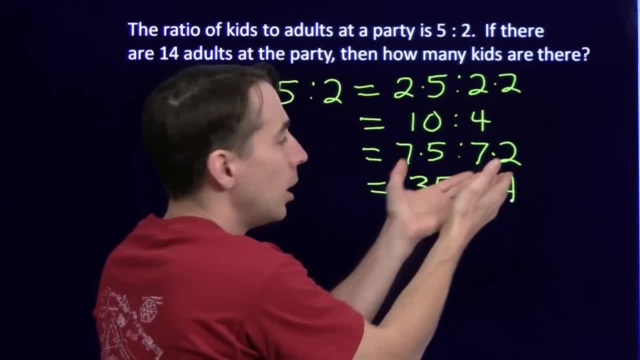 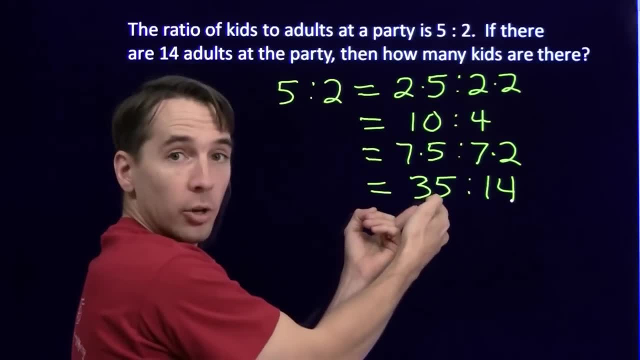 here is: we're taking the ratio, we're multiplying both parts of the ratio by the same number, and that gives us an equivalent ratio. We found a ratio here that has 14 adults. That's what we need, So the other part is the kids. It's 35.. Now, this is just one way to think about ratios. 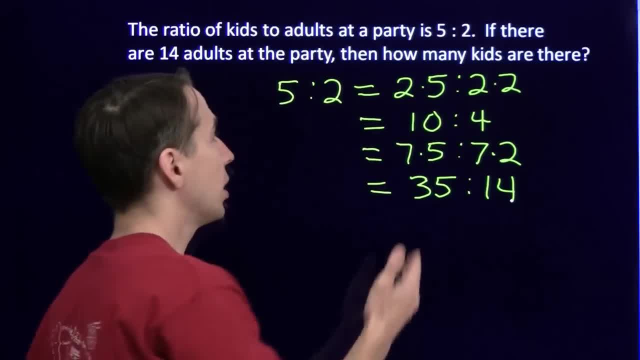 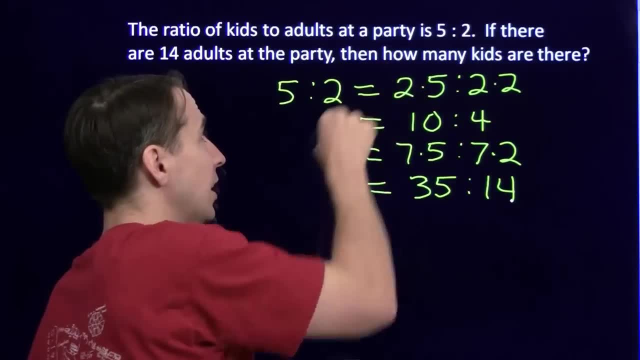 We're going to see a lot of different ways to think about ratios. One other way to think about this is if we have 5 to 2 kids to adults, that means in every group we can put them in groups. we'll have 5 kids and 2 adults. Now imagine we have x of these groups If 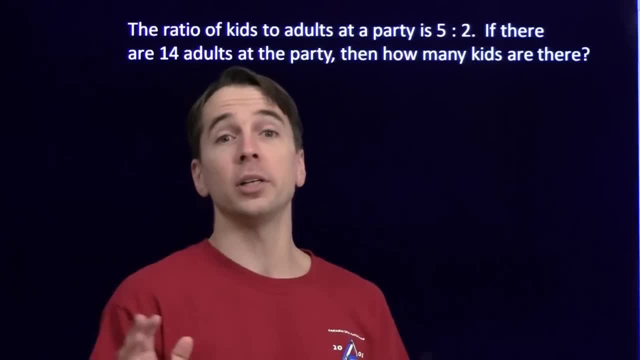 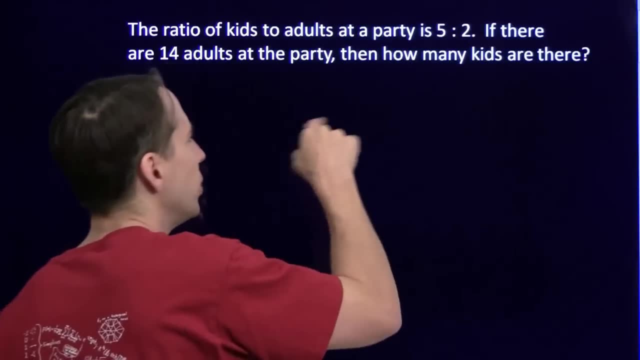 are. It just tells us that for every 5 kids there are 2 adults. We can put everyone in the party in groups and each of those groups will have 5 kids, 2 adults. That's all this ratio tells us. It doesn't tell us how many groups there are. Let's read the rest of the 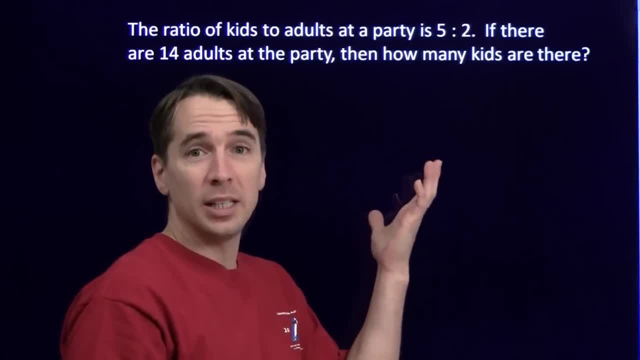 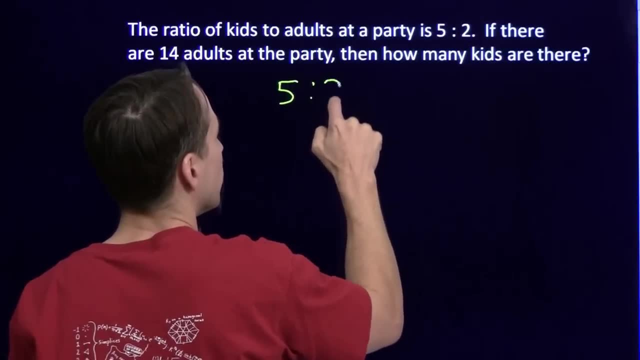 problem here. It says: if there are 14 adults at the party, then how many kids are there? So our ratio here tells us that we have 5 kids for every 2 adults. We could just have 5 kids and 2 adults, and that's it. Or we could have 2 of those groups If we had 2. 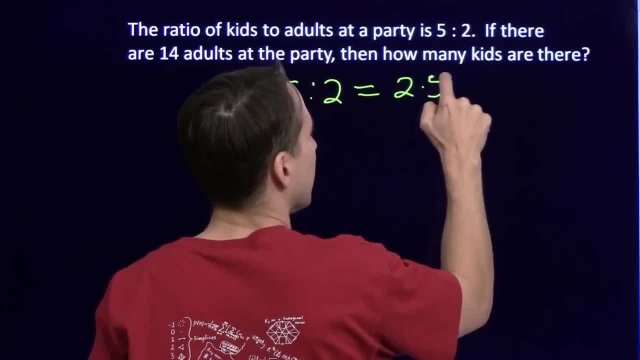 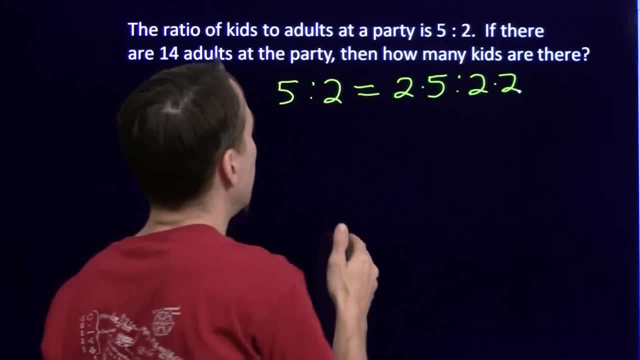 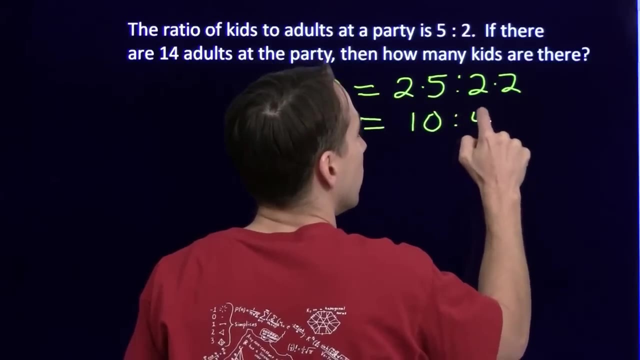 of those groups. well then, we'd have 2 times 5 kids and 2 times 2 adults, And all we're doing here is multiplying each of these components, each of these parts of the ratio, by 2.. So if we had 2 of these groups, that will give us 10 to 4.. 10 kids, 4 adults. 4 isn't 14.. 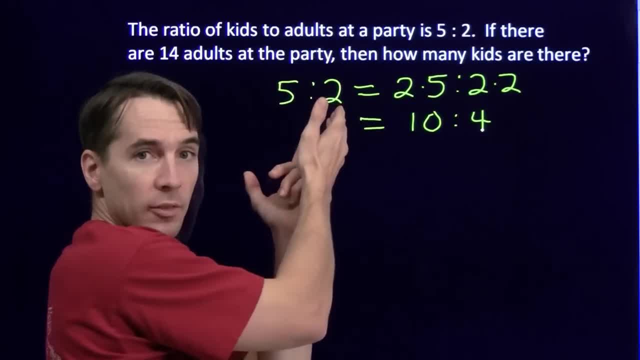 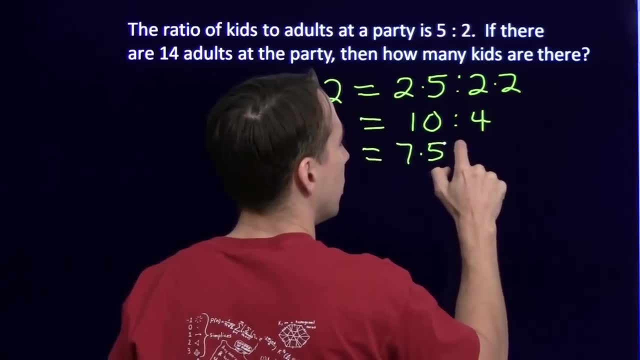 In order to get to 14 adults. well, we need 7 of these groups, 7 of these groups of 2.. So we can take a group of adults and we're going to multiply each of these groups by our ratio And again, multiply both parts by the same number. Multiply them both by. 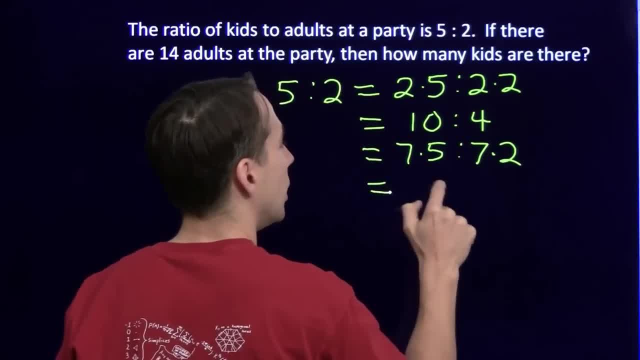 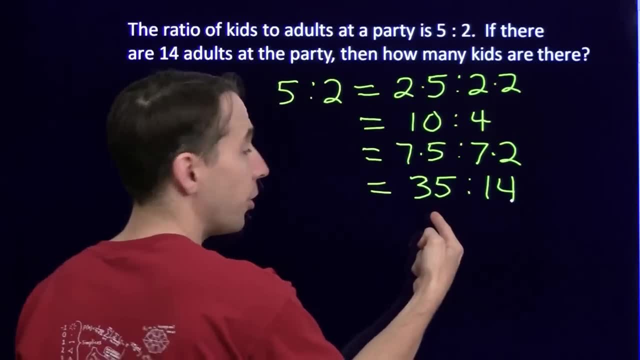 7. now It's like taking 7 of these groups and we get 35 to 14.. 14 adults, 35 kids. So we've answered the problem. We know there are 35 kids at the party And what we're doing. 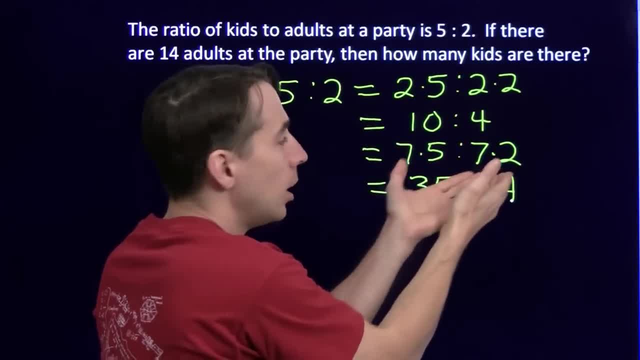 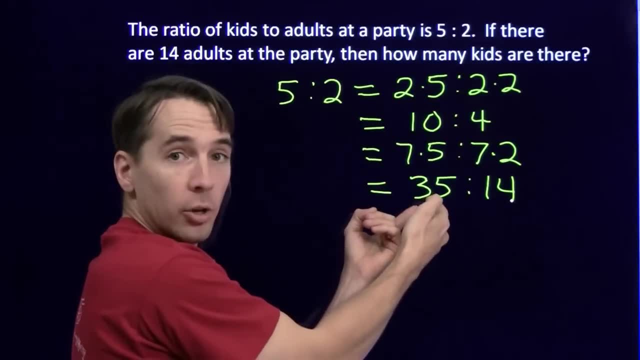 here is: we're taking the ratio, we're multiplying both parts of the ratio by the same number, and that gives us an equivalent ratio. We found a ratio here that has 14 adults. That's what we need. So the other part is the kids. It's 35. And this is just one way to think about ratios. 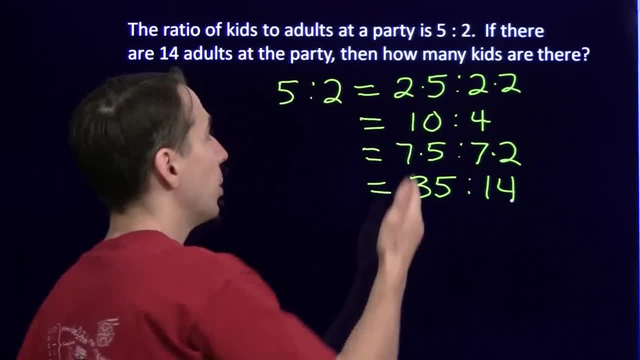 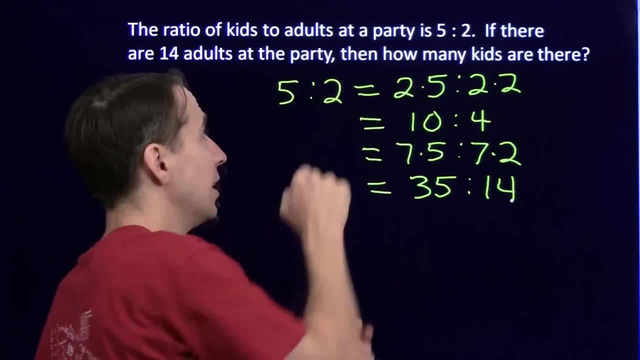 We're going to see a lot of different ways to think about ratios. One other way to think about this is if we have 5 to 2 kids to adults, that means in every group we can put them in groups. we'll have 5 kids and 2 adults. Now imagine we have x of these groups If 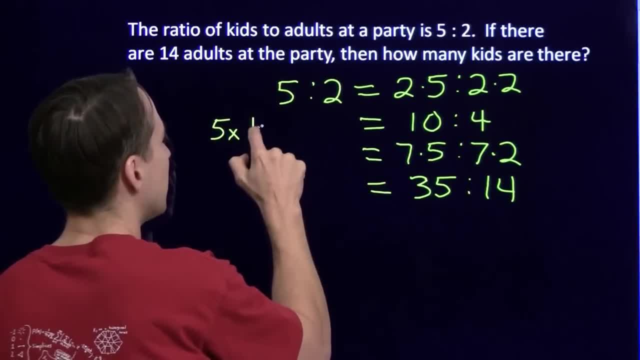 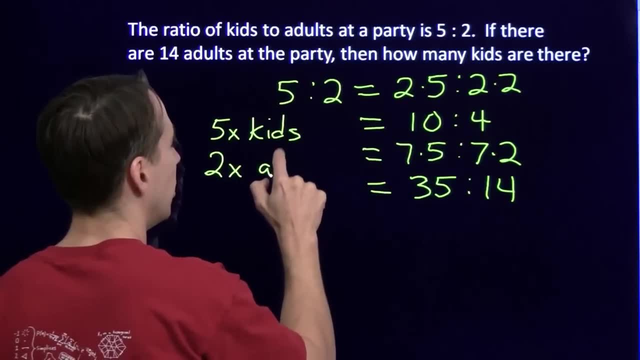 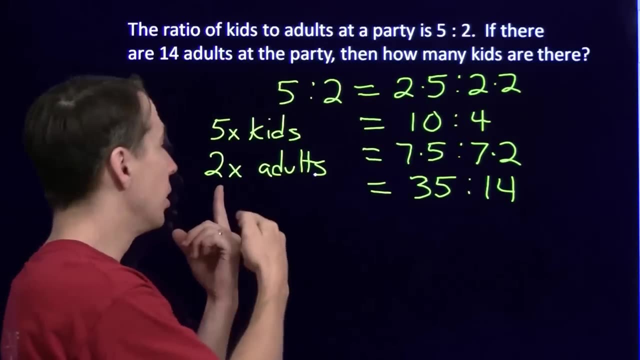 we have x of these groups, then we have 5x kids, because there are 5 kids in each of these groups And we have 2x adults And once again 2x equals 14. That means x is 7. Put 7 in here. 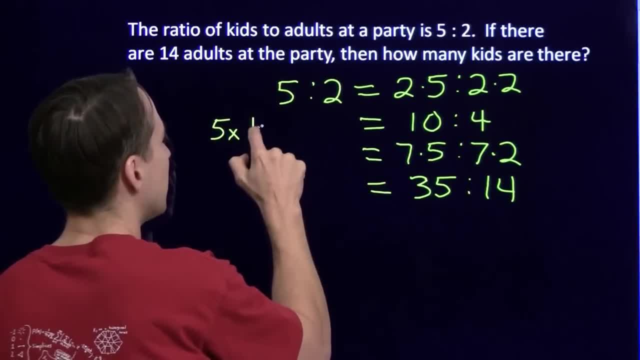 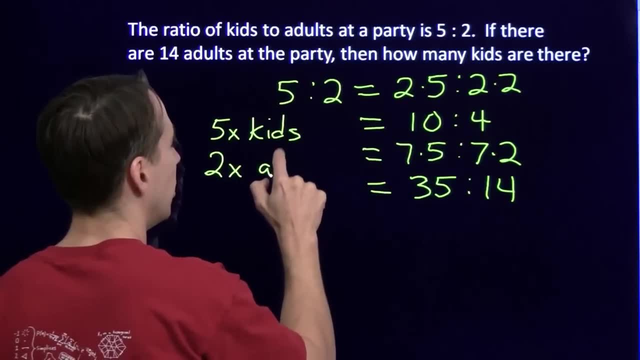 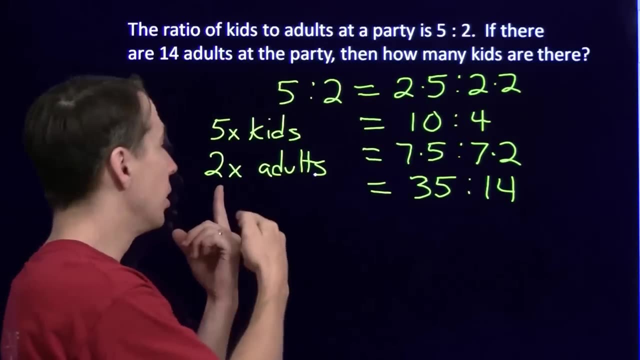 we have x of these groups, then we have 5x kids, because there are 5 kids in each of these groups And we have 2x adults And once again 2x equals 14. That means x is 7. Put 7 in here. 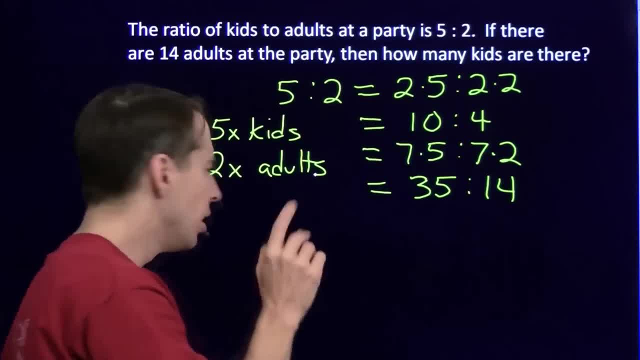 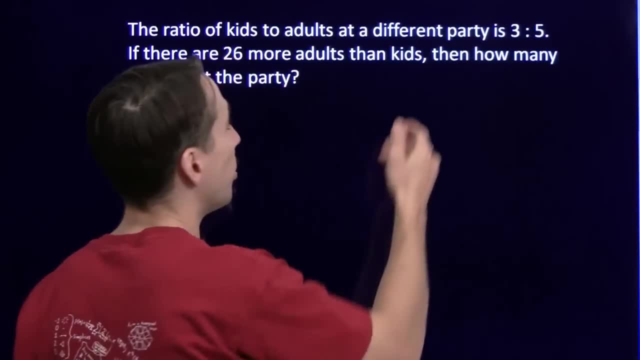 5 times 7 is 35. We get 35 kids once again. Let's take a look at another ratio problem. Here we have kids to adults at a different party. The ratio is 3 to 5. That means for every 3 kids there are 5 adults. This is. 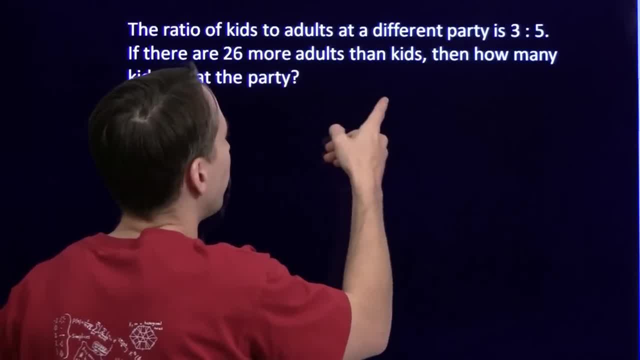 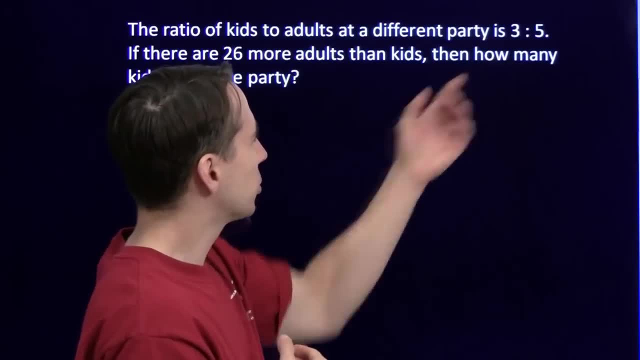 going to be a boring party. Ah, But there are 26 more adults than kids. Then how many kids are at the party? Let's approach this like we did in the first problem. Just think about these groups here. In each group, we have 3 kids and 5 adults. 3 kids and 5 adults. That means each of these. 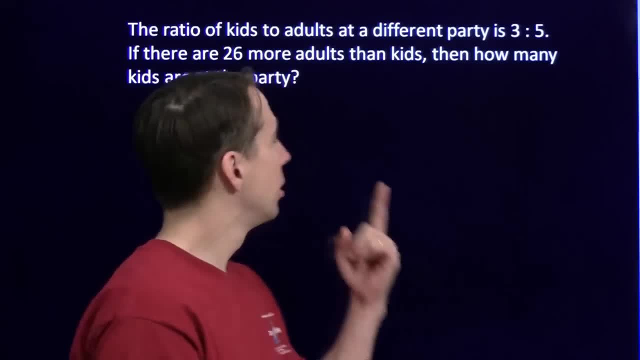 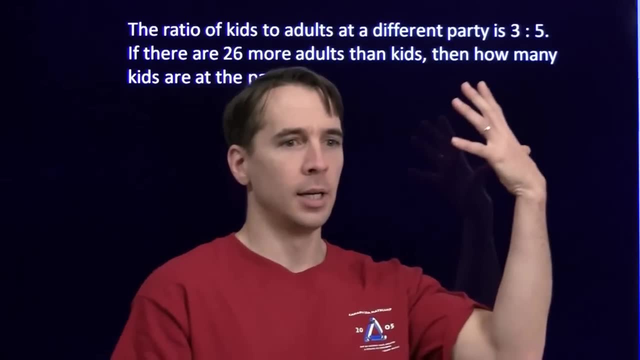 groups has 2 more adults than kids. Now, in total I need 26 more adults, But one of these groups has 2.. So if I had 2 of these groups, that would give me 6 kids and 10 adults. That difference would be 4.. 3 of these groups. 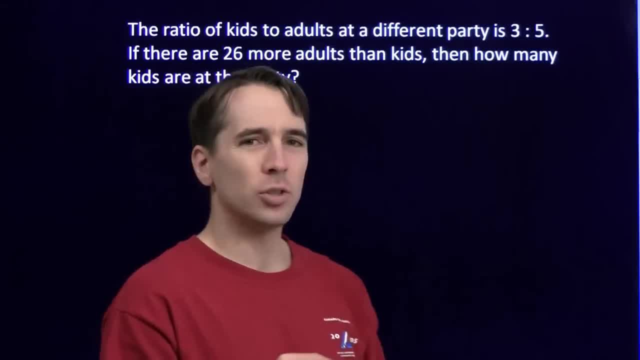 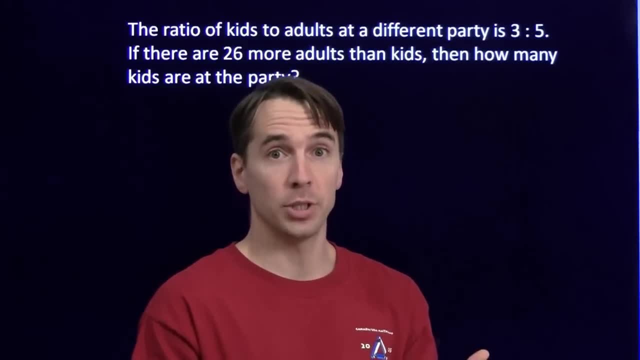 the difference would be 6, 4 of these groups, and so on. So in each of these groups I have 2 more adults than kids. I need a total of 26 more adults. That means I need 13 groups, 13 of these groups. 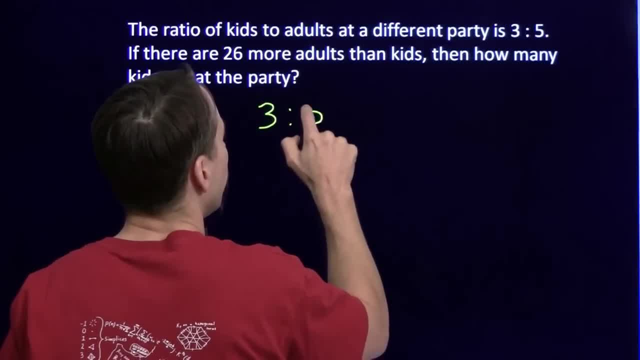 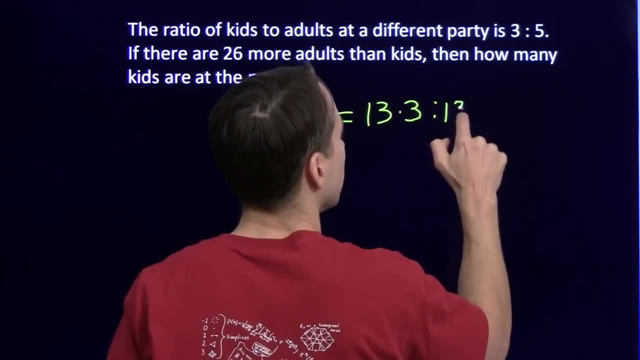 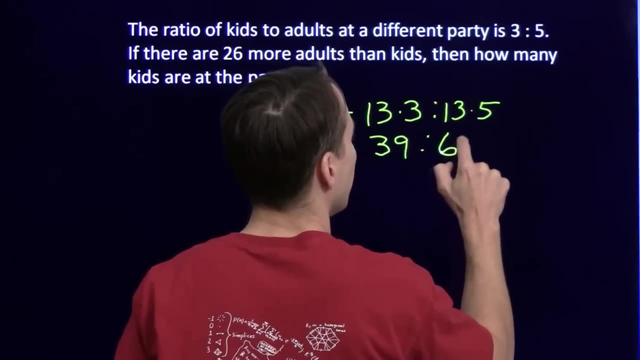 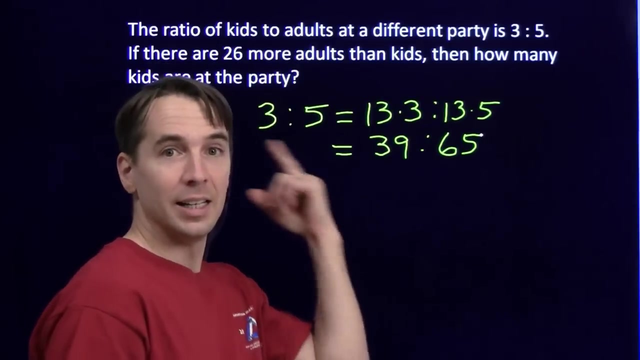 Let's check that and make sure we did that right. 3 to 5.. If I have 13 of these groups, I multiply both parts by 13.. 13 times 3 is 39.. 13 times 5 is 65. Sure enough, 65 is 26 more than 39. So there are 39 kids at the party. 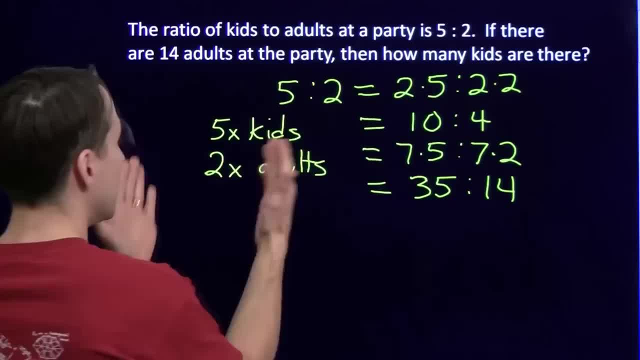 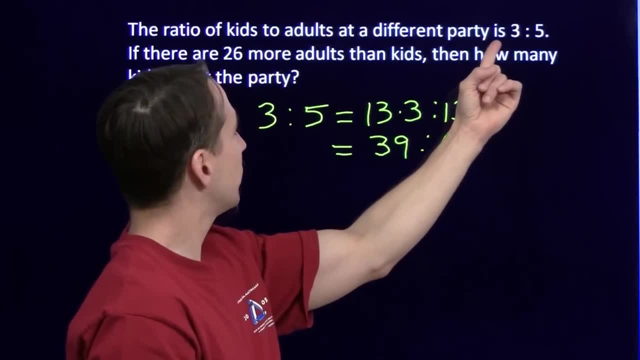 Now another way we can do this. let's go back and look at the second way, The second way we did this problem putting in the x. we'll come back to our second problem. Our ratio of kids to adults is 3 to 5, and we have, say, x of these groups. That means we have 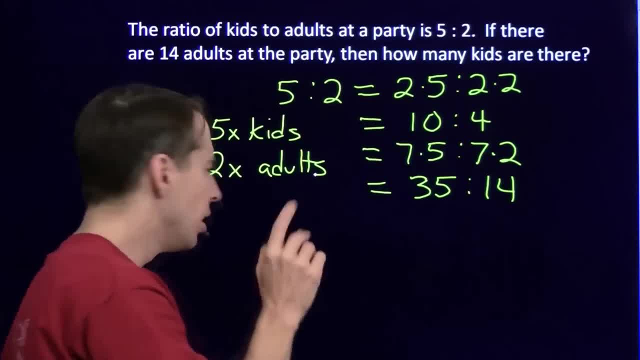 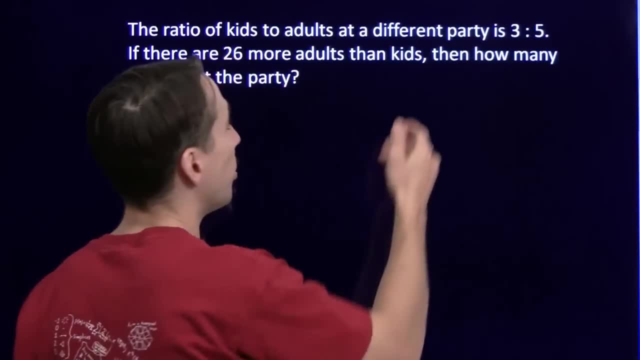 5 times 7 is 35. We get 35 kids once again. Let's take a look at another ratio problem. Here we have kids to adults at a different party. The ratio is 3 to 5. That means for every 3 kids there are 5 adults. This is. 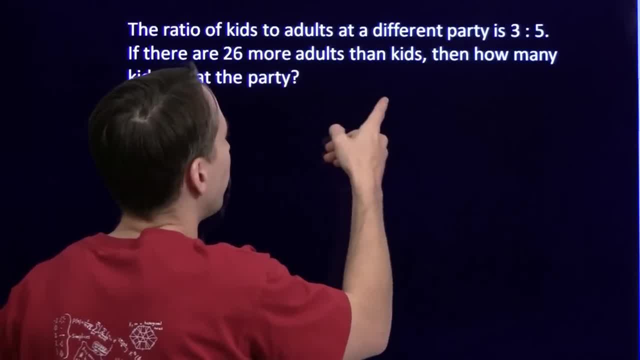 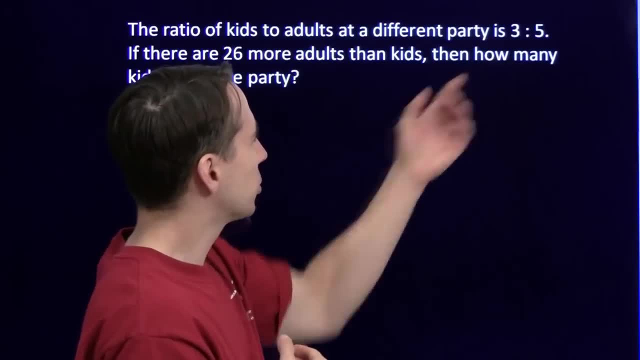 going to be a boring party. Ah, But there are 26 more adults than kids. Then how many kids are at the party? Let's approach this like we did in the first problem. Just think about these groups here. In each group, we have 3 kids and 5 adults. 3 kids and 5 adults. That means each of these. 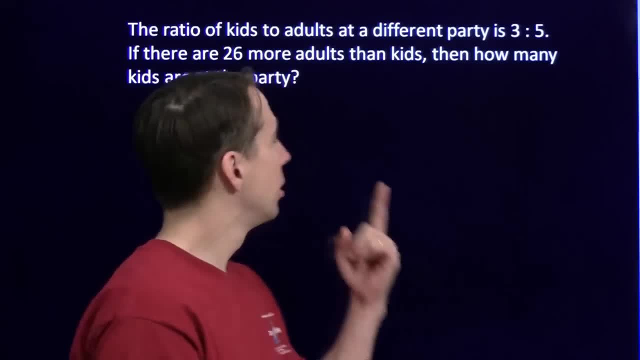 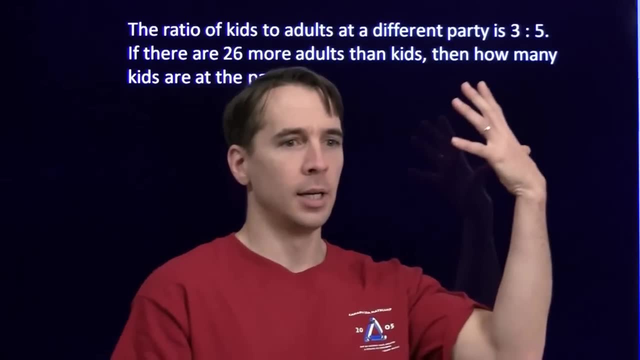 groups has 2 more adults than kids. Now, in total I need 26 more adults, But one of these groups has 2.. So if I had 2 of these groups, that would give me 6 kids and 10 adults. That difference would be 4.. 3 of these groups. 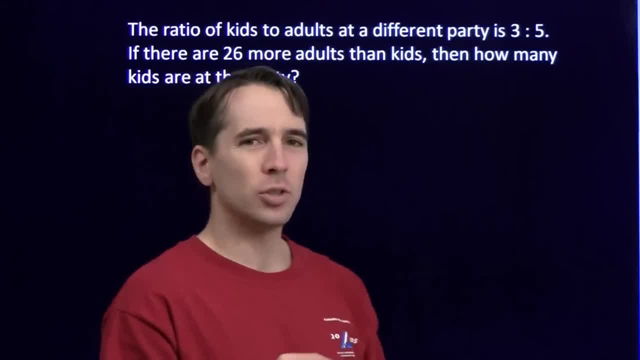 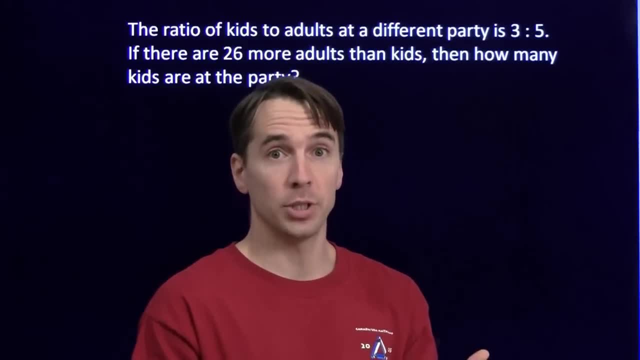 the difference would be 6.. 4 of these groups and so on. So in each of these groups I have 2 more adults than kids. I need a total of 26 more adults. That means I need 13 groups. 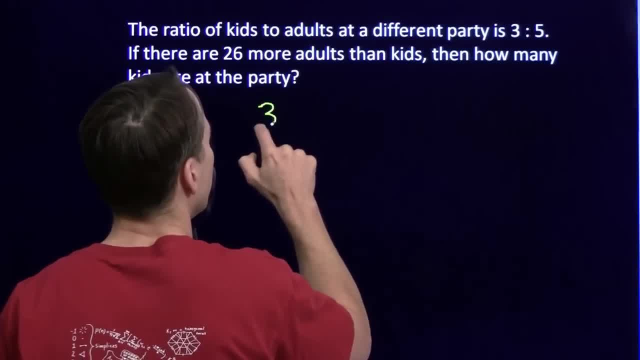 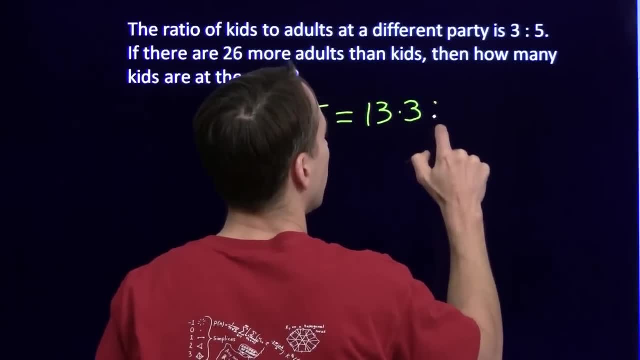 13 of these groups. Let's check that. Make sure we did that right. 3 to 5.. If I have 13 of these groups, I multiply both parts by 13.. 13 times 3 is 39.. 13 times 5 is 39.. 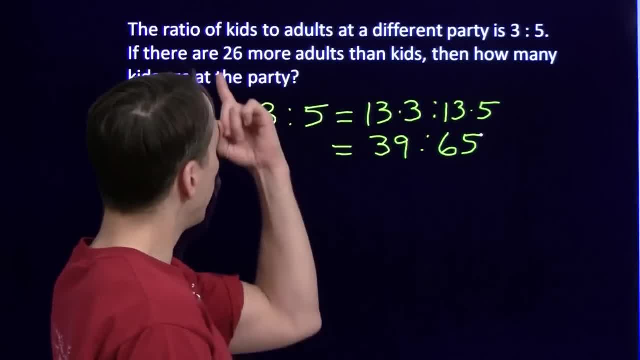 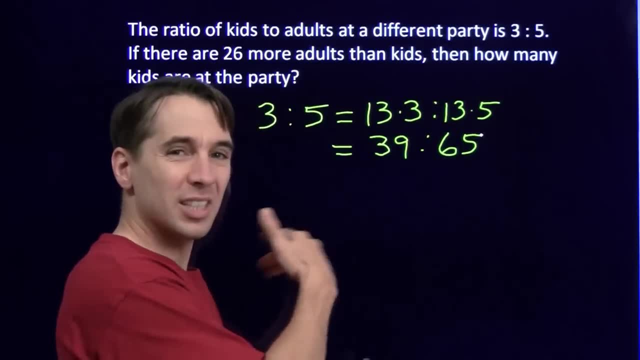 35 times 8 is 65. Sure enough. 65 is 26 more than 39. So there are 39 kids at the party. Now, another way we can do this: let's go back and look at the second way. The second way. 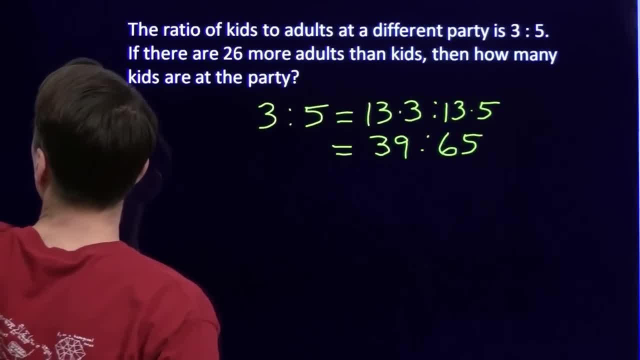 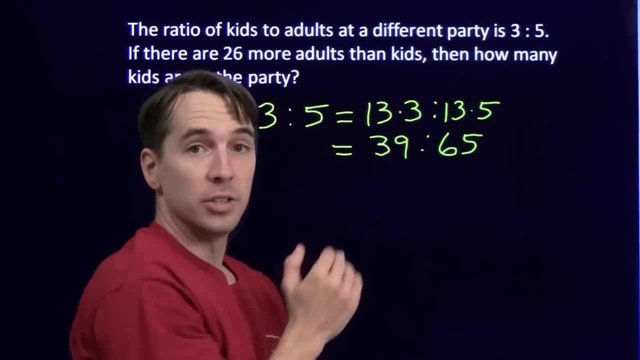 we did this problem putting in the x. We'll come back to our second problem. Our ratio of kids to adults is 3 to 5. And we have, say, x of these groups. That means we have 3 x kids. 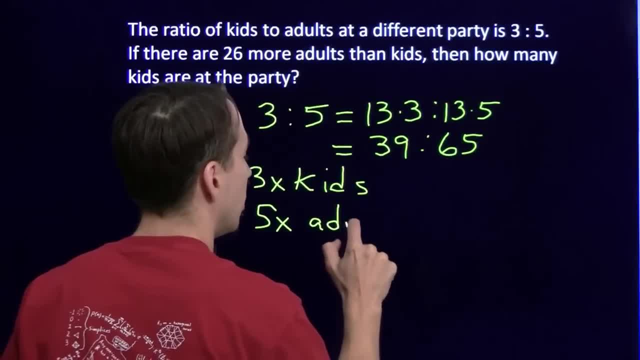 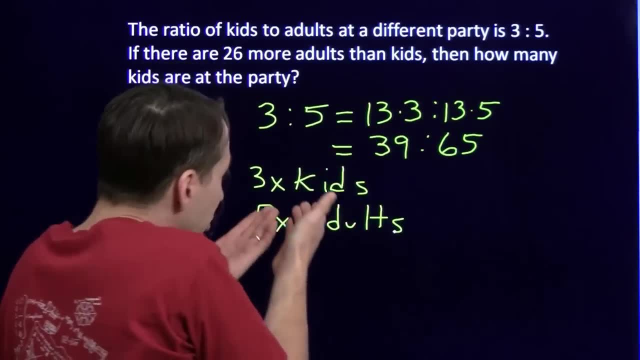 And 5 x kids. Again, that's just because we can take this ratio and make an equivalent ratio by multiplying it by any number. Up here we multiplied it by 13,. down here we're multiplying it by x And what we're told is that there are 26 more adults than kids.